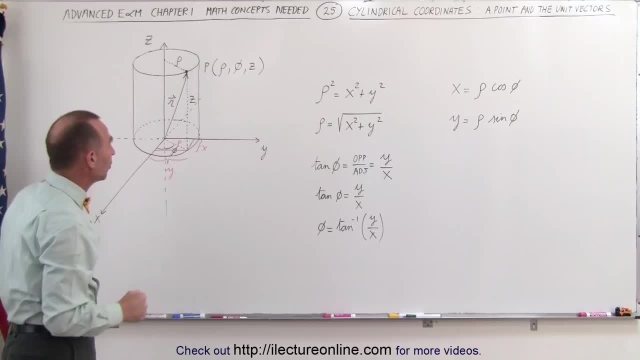 Relating that to the Cartesian coordinate system, to the XYZ coordinate system, you can see that rho squared is equal to x squared plus y squared, because this is simply a triangle. This here would be x, this here would be y, this here would be the hypotenuse rho. So rho squared equals x squared plus y squared, And maybe I should put x over here, So this could be considered x, this could be considered y, And there's your right triangle right there, And there's the angle phi. 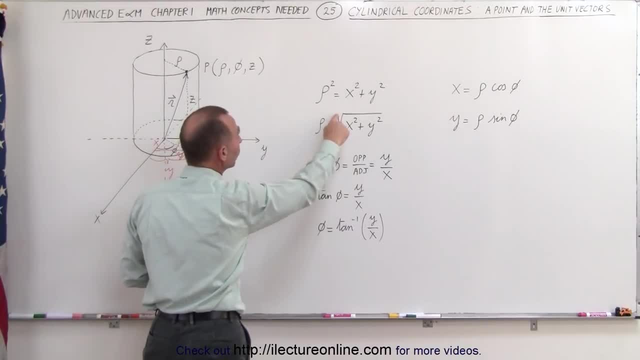 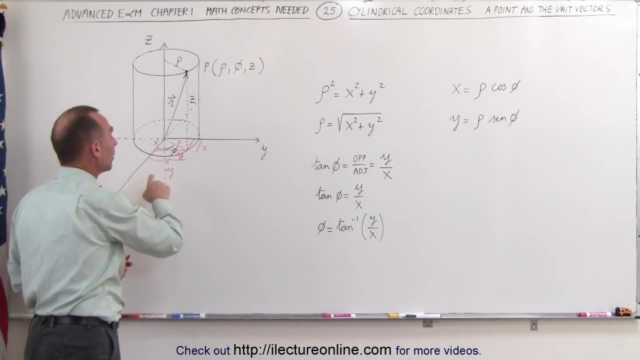 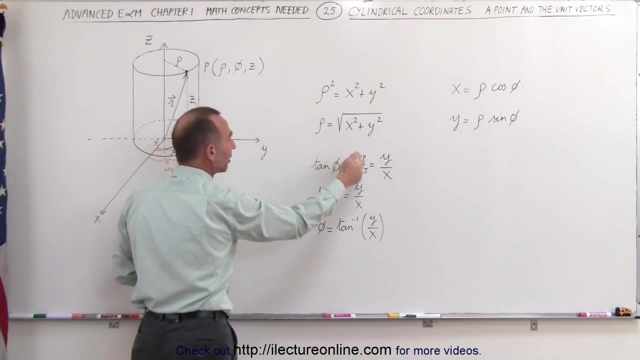 Then you can solve for rho. Rho is equal to the square root of x squared plus y squared, Relating the tangent or relating the angle phi to x and y. we can simply take the tangent of the angle. The tangent of the angle is determined or defined by the opposite side, divided by the adjacent side. 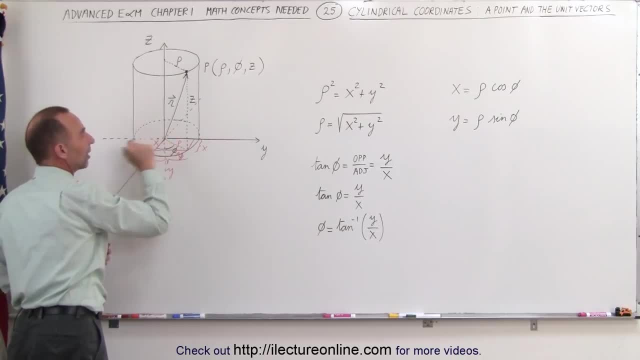 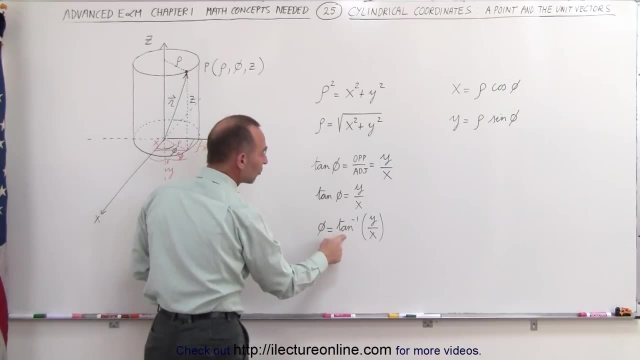 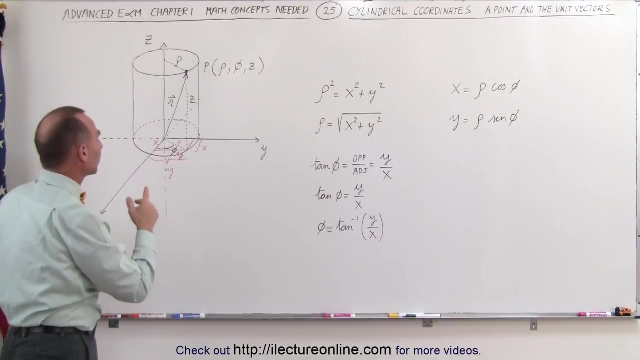 The opposite side to the angle is y. The adjacent side here is x. So therefore, the tangent of phi is y over x, And theta can then be defined as the r-tangent. So this is the tangent of y over x. Finally, we also want to be able to convert from the or. we want to be able to express x and y in terms of the cylindrical coordinates. 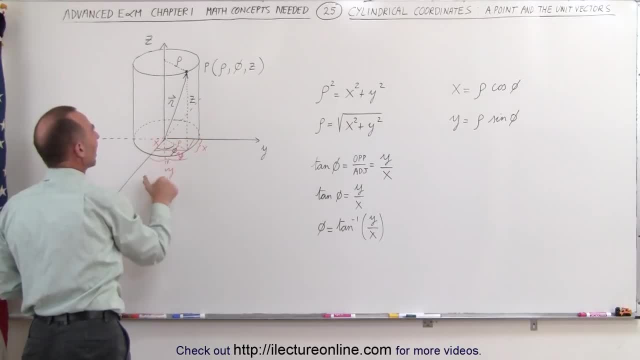 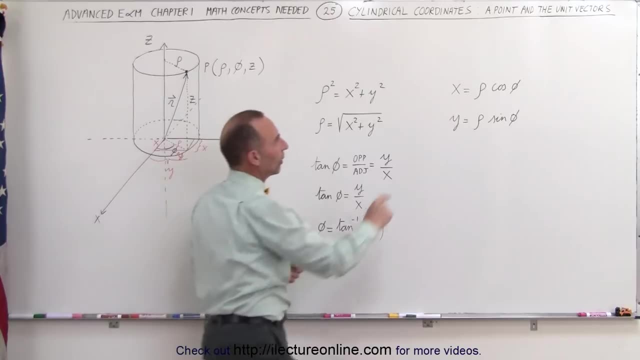 And if you look at x here, x can be defined as the hypotenuse rho times the cosine of the angle, because the cosine represents the adjacent side. So x can be defined as rho. the distance from the z-axis to the point times the cosine of phi. 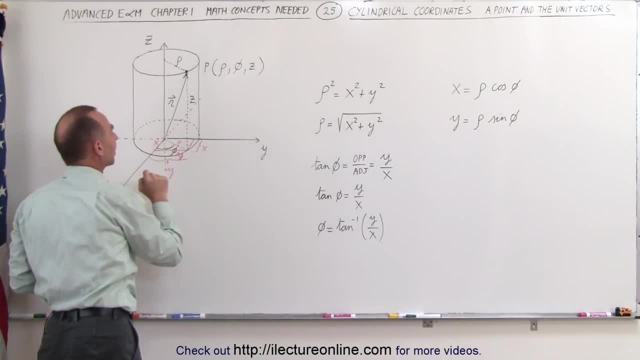 And then y. y is the tangent of the angle phi, the opposite side to the angle. therefore, y can be defined as a hypotenuse rho times the sine of the angle phi. And that's how we go back and forth between Cartesian and. 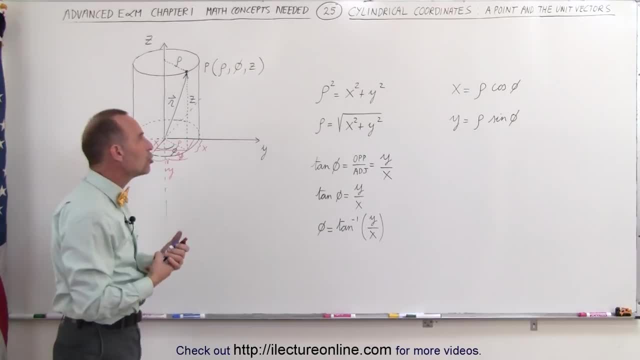 cylindrical coordinates. Now we also want to talk about the unit vectors. The unit vectors in the Cartesian coordinate system is x-hat, y-hat and z-hat, or i, j and k as we know it. So what are the unit vectors and what are the directions of the unit vectors in? 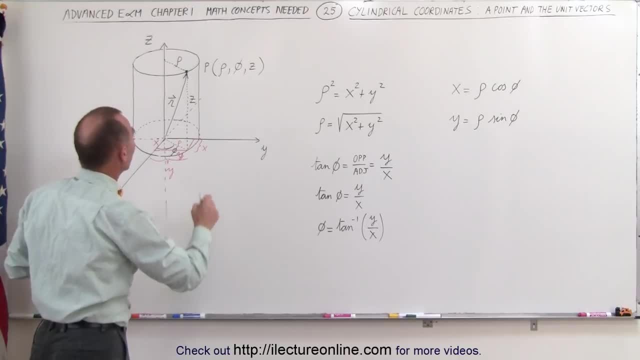 cylindrical coordinates. Well, first of all, the unit vector for rho is simply straight out in this direction. So, again, it goes from the z-axis to the point, and then we draw a unit vector in this direction, and this is then known as the rho unit vector. The